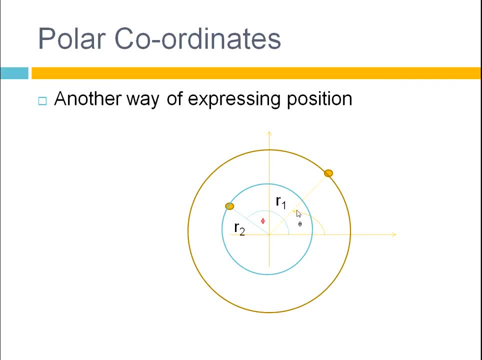 Say, this circle is r1, and you can go round by theta and trace out all the points in that circle. So by varying the radius of a circle and going round all of the angles you can get all of the points, An infinite number of points. 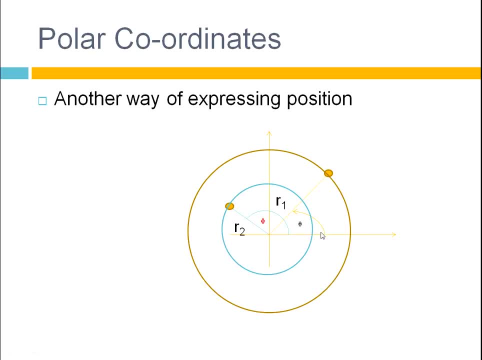 So any point can be expressed using these two parameters. This is polar coordinates And when we think about the circles, you can define any position on the circle in the rectangular coordinates, which is x and y's, to be x equals r cos theta and y equals r sin theta. 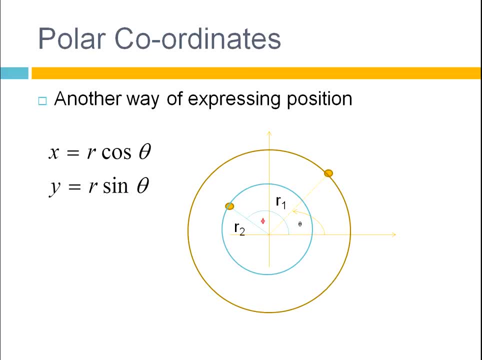 And when you think about this it actually does make sense. Think about this point here. This is theta equals 0 on this gold circle. So if we put theta equals 0 into this, cos of 0 is 1.. So x is just r. 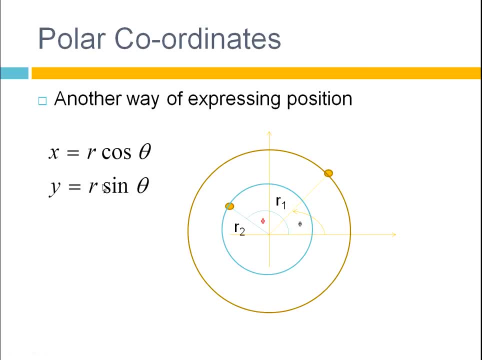 And sin of 0, you should know, is 0. So y equals 0. That point. there is point r0. And you repeat this for any point on the circle and it will convert between polar to your rectangular normal xy coordinates. If you remember, a complex number is written: z equals x plus iy. 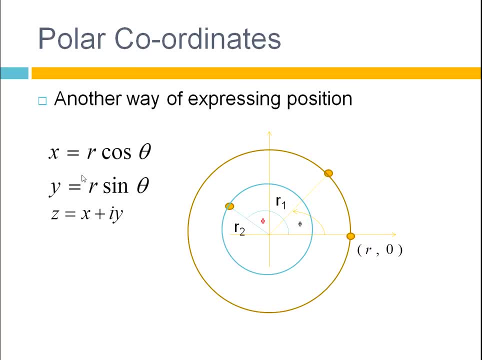 So if you substitute this and this into your x plus iy, like so x is r cos theta That goes in there, y is r sin theta That goes in there, You get this expression here, which is exactly the expression on the previous slide. 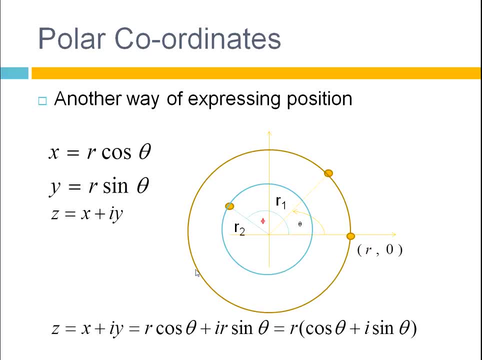 This is your polar coordinates, And this can also be written in other ways. You sometimes see it as r cis theta, where the cis is just cos i sin, cos i sin, which is pretty unoriginal. Or you can just write it in an even shorter form: 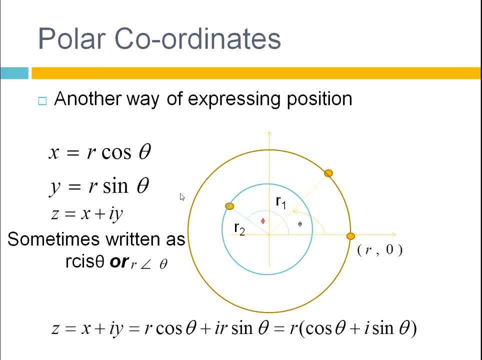 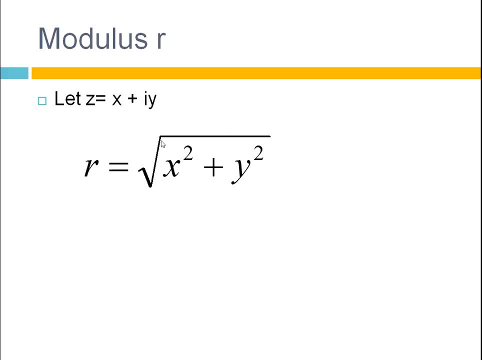 which is r, at an angle theta. So we're going to look at how to find the modulus r. It's very simple. It just comes from Pythagoras. You get this expression here If you draw out a point. it's quite obvious. 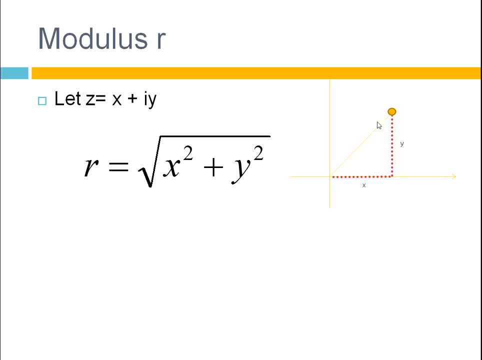 You go along by x, You go up by y, And the length of this is just going to be this expression here. So if you had z equals 3 plus 4i, where this here is your x and that there is your y. 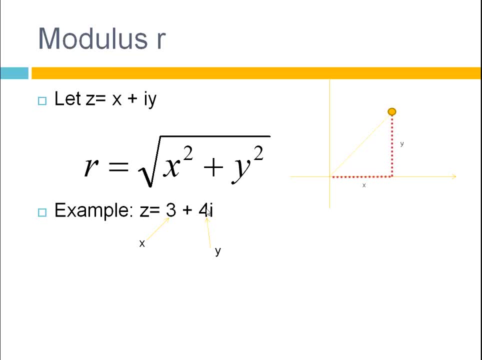 that's only the 4,, not 4i, just the 4.. That's your coefficient, So you have to look there. Just the coefficient of i is the value of y, So put that in here, You get 5,. 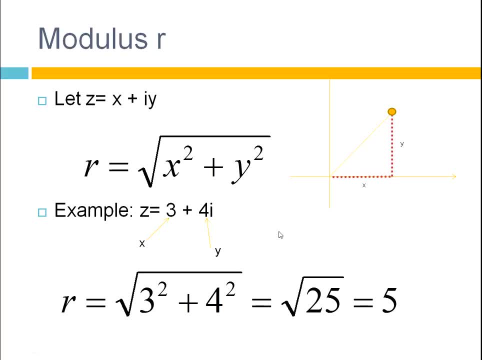 which is quite obvious: 3 squared plus 4 squared is 5.. Now we find the argument slightly more difficult. You've got the same example: z equals 3 plus 4i, And the formula is tan. theta equals y over x. 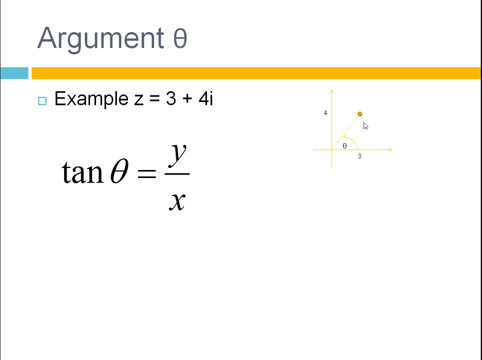 Now always draw a diagram, Just plot the point. Make sure that the value of theta is a reasonable value, So we'll work it out. You get tan. theta equals 4 over x Equals 4 over 3.. If you take the inverse tangent, 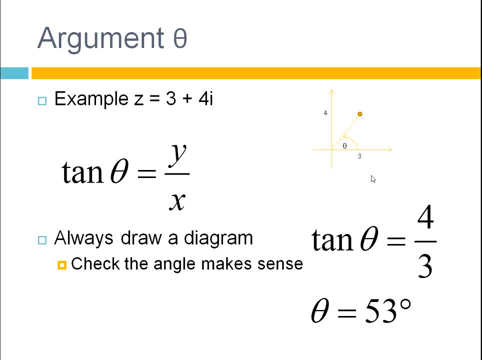 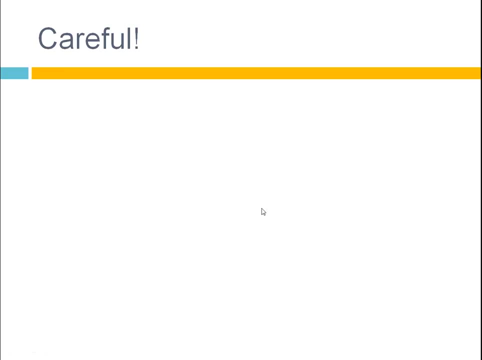 you get. theta equals 53 degrees. Look back at the diagram. Does 53 degrees look like a reasonable angle? Obviously, this is between 0 and 90. So 53 is quite possible. Alright, So let's look at the ones where the diagram is even more helpful. 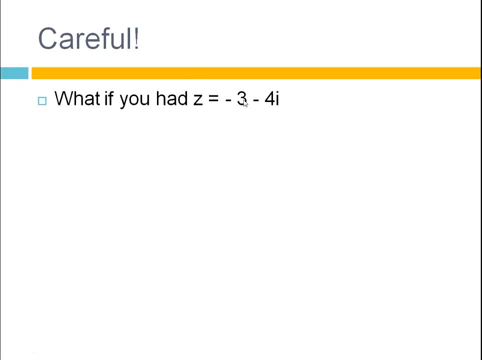 Say you had a very similar example, but with the negatives in here. So you're at: z equals minus 3 minus 4i. If you work out the argument, you get exactly the same answer as the previous question, Because the minus is cancelled. 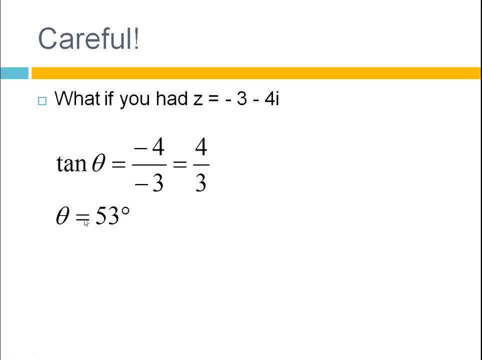 so it's just the same. That's 53 degrees. So if you draw it out like that, that angle is obviously not going to be 53 degrees, So you need to do a little calculation. So 180 plus 53 gives you 253.. 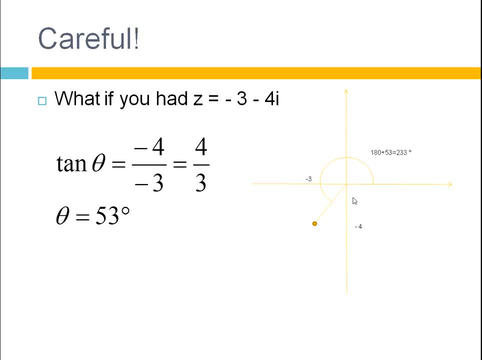 That does look like 233 degrees. So you've got 180 going round there and then you've got your 53 degrees in here. Strictly speaking, the 53 degrees that you got would be a kind of reflection of this. So the line up there. 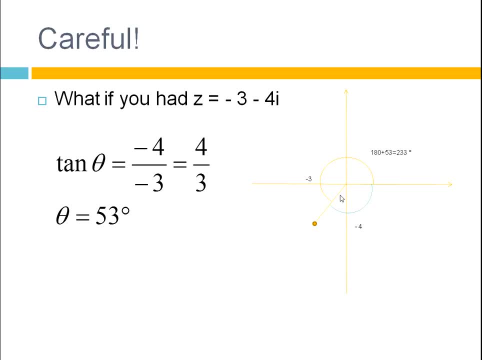 So you've got a 53 round there which corresponds to that angle. You can also find the negative angle which is going round in the opposite direction, Which is just minus 90, minus this thing in here. You've got minus 90 going round that way. 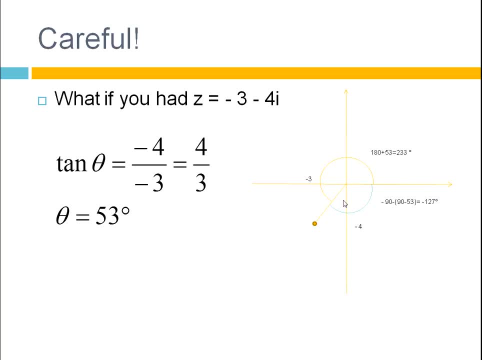 And you want to find this angle in here, which is just 90 minus 53.. 90 going all the way round here, Less this bit in here. You can see that there. You just add that up. Remember it's the negative direction. 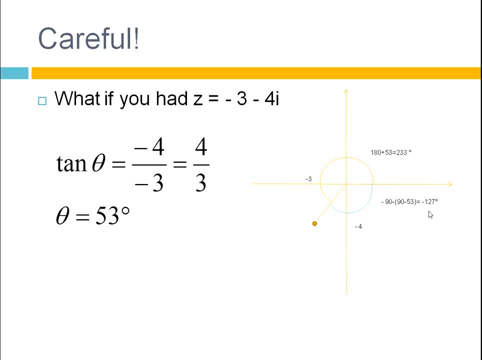 This minus 127. And these obviously add up to 360 all the way round. And you can express it using either of those: The plus or minus angle, It doesn't make any difference. So I'll do a full example. to find the root 2 minus i root 2 in polar form. 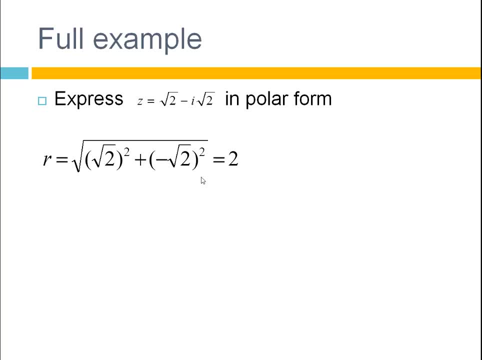 Exactly the same steps And find the modulus as. so: Just your x squared plus y squared, And when you square something with a negative it just becomes positive. 2 plus 2, square root is 2.. And finding the argument, Remembering to draw a diagram. 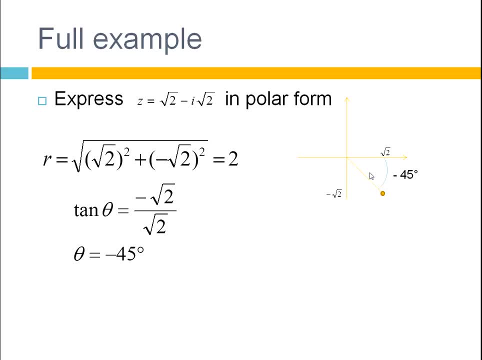 The argument is minus 45, which is obviously this angle going round this way. Negative angles are going round like that And you can also mark out the positive angle. It's going to be 315.. 360 degrees all the way round. 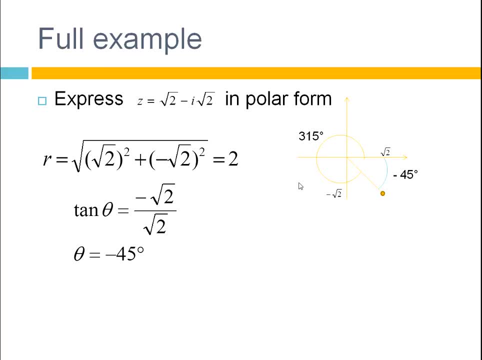 Less than 45 degrees there. So you plug that into the r cos theta plus i sin theta. It's your expression for polar form. You get this. I've used the positive angle here for the 315.. And there's other ways you can express this. 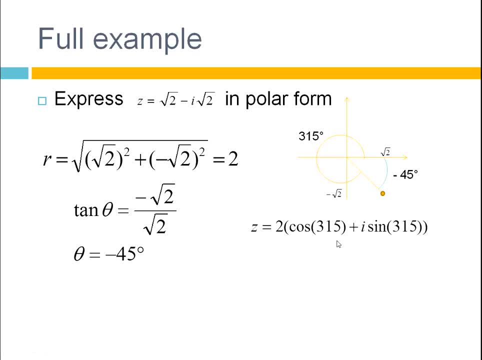 It's what's called Euler's identity, Which is just r, e, i, theta, Just like that. And then there's the very lazy short form, Which is just the modulus at an angle. So that's how you write out a number in polar form.